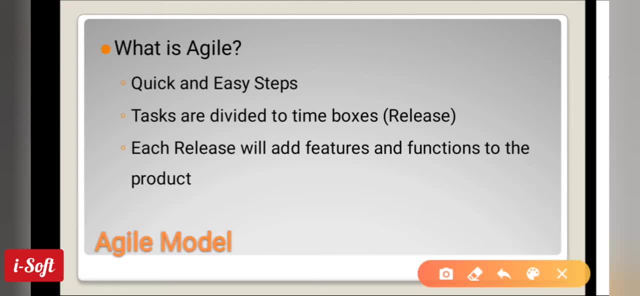 into different modules, and in each module we will add some or more functionality into that software. and hence at the last, after when we will complete all development of modules, we will get the complete working project. So hence the tasks are divided into time boxes, or release, or iteration, We will call it as time. 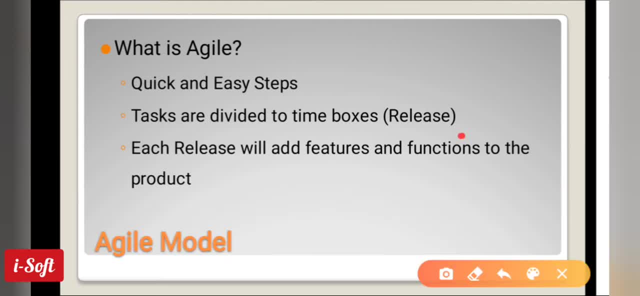 boxes or release or iteration. So in each iteration we will add up some functionality into that software. Hence, each release will add features and functions to the product. Each release we will, we will update the product Each release. so hence, agile means simply what is agile? Agile means: 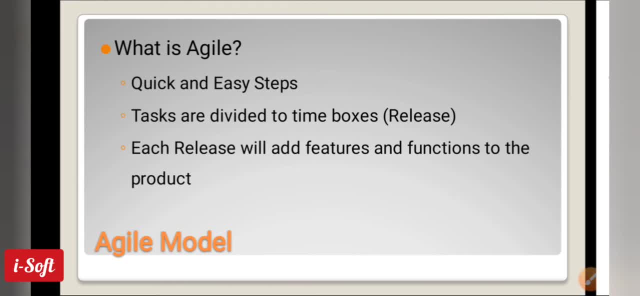 quick and easy steps, or agile means dividing the complete procedure into different number of iteration, and in each iteration we will add up some functionality into the software. iteration by iteration we will continue the development. So hence, what is agile model now? So in agile model, 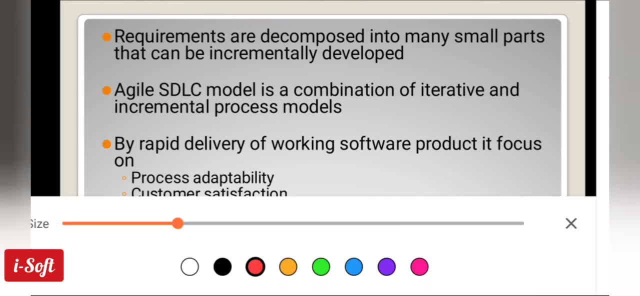 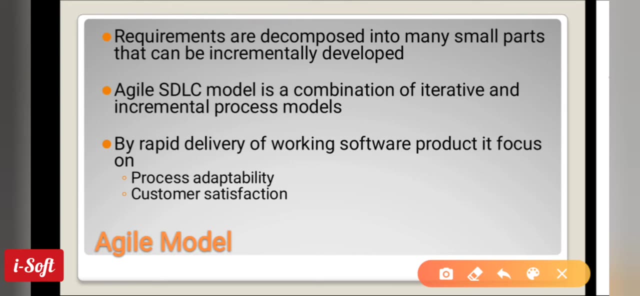 the requirements are decomposed into many small parts. So the requirements are decomposed into many small parts and hence in each iteration we will work on different requirements that are functional or non-functional requirement in SDLC and in waterfall also. we have discussed very much about the requirements. 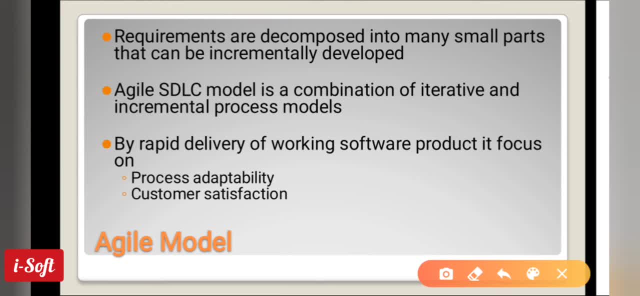 So the requirements are gathered and then that requirements are decomposed or divided into many number of small parts, and in each iteration we will develop this one of the part of this requirement which are decomposed Then in agile SDLC model. it is a combination of iterative and 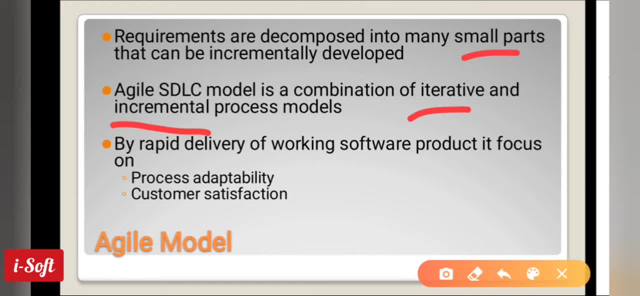 incremental process models. What is iterative process model? Iterative process model means in iteration by iteration we will develop our software and in each iteration we will add up some functionality into that software. And in incremental process, incremental process means we will add up some functionality in 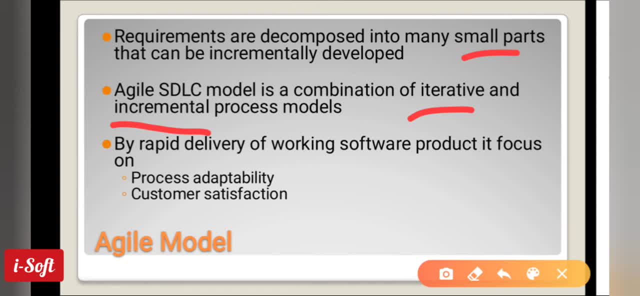 each step. hence we will go incrementing the requirements or functionality of the software. hence it is called as incremental model or incremental process, and this agile model. agile model is the combination of iterative and incremental process. models means iteration. by iteration we will develop and also in each iteration we will add up some functionality. 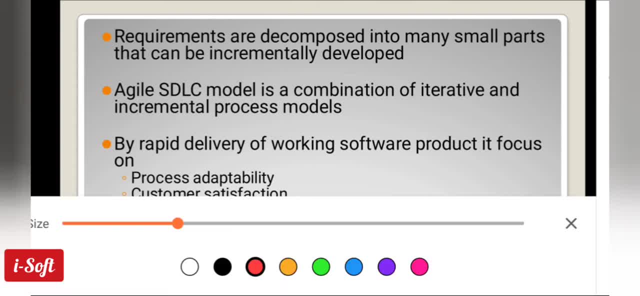 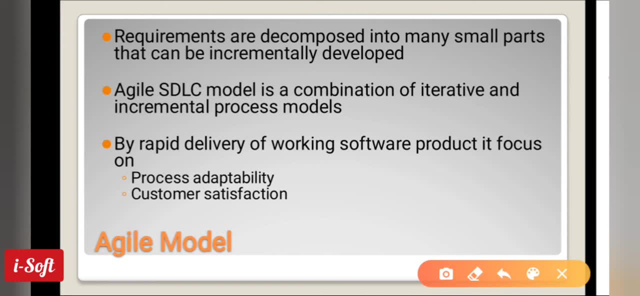 into the software or into the product. So by rapid delivery of working software product it is focused on. so what it means? it is focused on product adaptability, adaptability and customer satisfaction. So if the product is developed, then that product must be adapted. 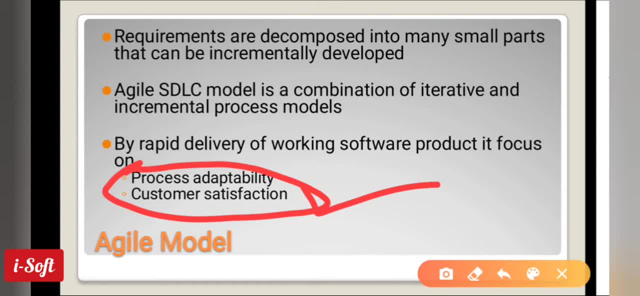 by the customer and also it is focusing on customer satisfaction. So how it will focus on this? customer satisfaction by rapid delivery of working software means as soon as first iteration is completed, the product is delivered to the customer and the product will be checked by the customer. So it is rapid delivery of working software. that software will be. 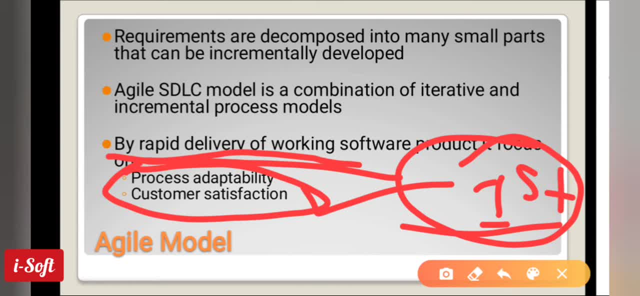 must be working software. definitely it will be working software. So first model will be delivered to the customer. and then, what are other requirements that are added? iteration by iteration, in various steps. So first model is delivered to the customer within 2 to 3 weeks. So each model will take 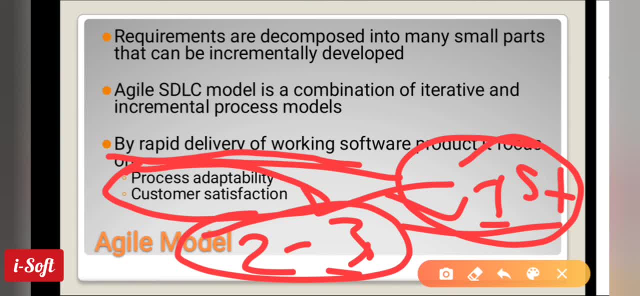 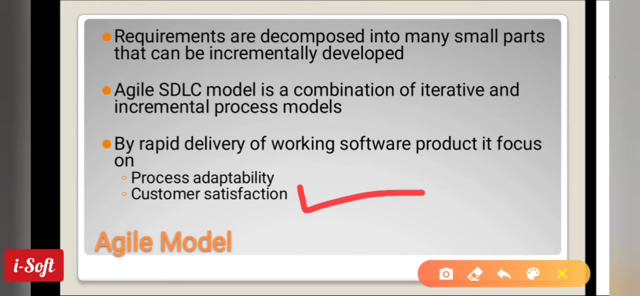 2 to 3 weeks to develop, So it is rapid delivery of working software. So how it is performed: by iteration, by iteration, and also it is focusing on product adaptability. the product will be adapted by the customer and customer satisfaction is important for agile model. Then next these: 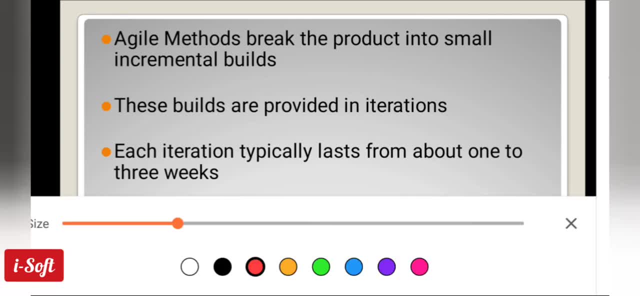 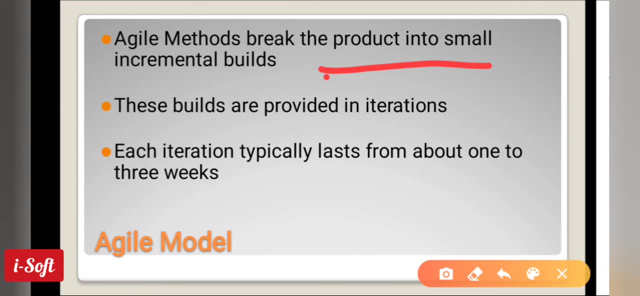 agile methods break the product into small integrations. So, as we have discussed already, the product is divided into small incremental iterations, or builds or release. it is called as small part of program. you can consider it as a small part of program. So these builds are provided in iterations. in each iteration we will develop. 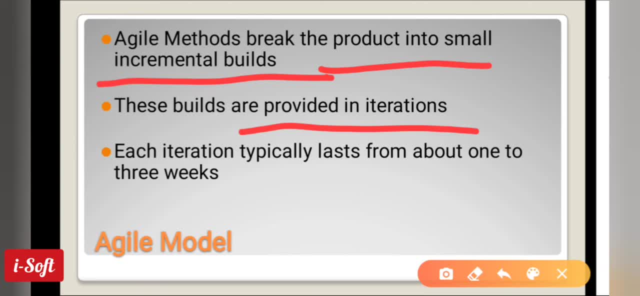 one build or one release of the software or one part of a program of software and each iteration. So these builds will be developed within 1 to 3 weeks, as we have discussed already: 1 to 3 weeks. within 1 to 3 weeks we will develop each of the build, and when we are developing, 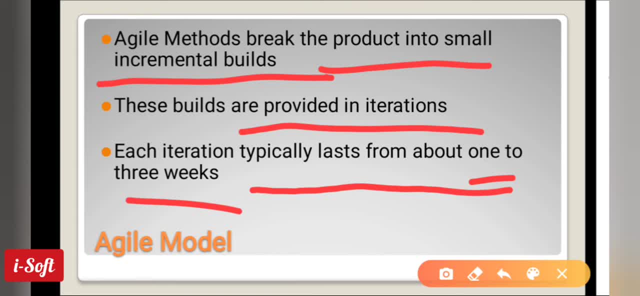 these builds. So, after developing first build, second build will add functionality into first build. then third build will add functionality into whatever is developed previously, whatever build is developed previously. So they are adding functionalities that are developed previously into the software that are developed previously. 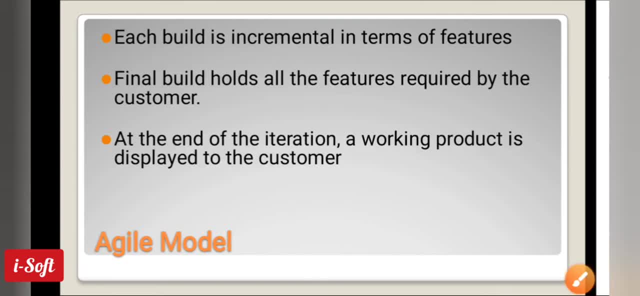 So next, each build is incremental in terms of feature. what it means each build is incremental in terms of feature means means each build will add or increment the functionality or feature of the software. So each build is incremental in terms of feature. then final build holds all the features that are required by the customer. This means this means the 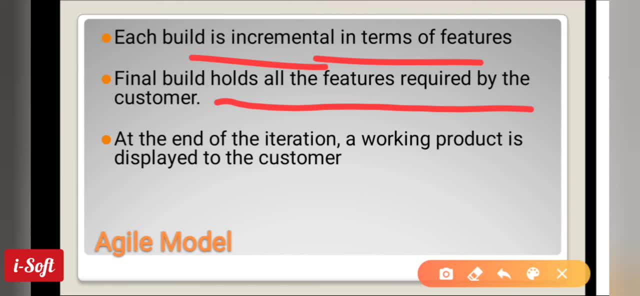 product will be developed into the final build. So each build is incremental in terms of feature means each build will add the functionality. the previous build and last build will be our final product. So, after completing all the iterations, our final product will be whatever. 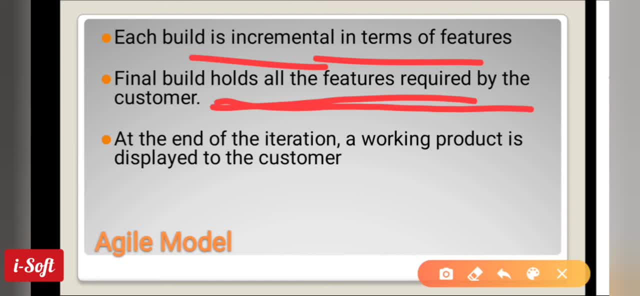 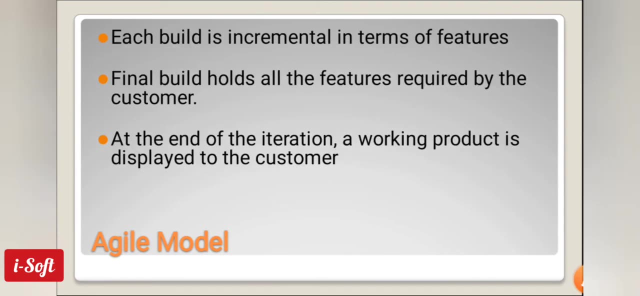 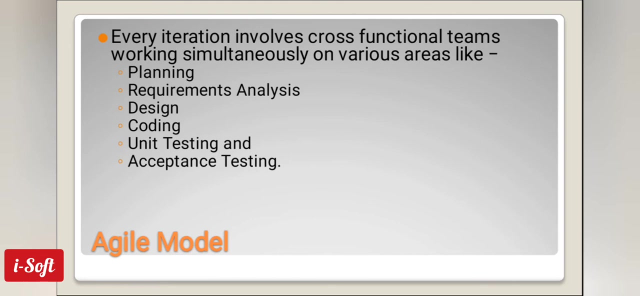 is developed in last build or last release or last part of the software which is developed is our final product. At the end of iteration a working product is delivered to the customer, displayed to the customer. so so each build is incremental build, so at last we will get the complete product. then every iteration involves cross functional. 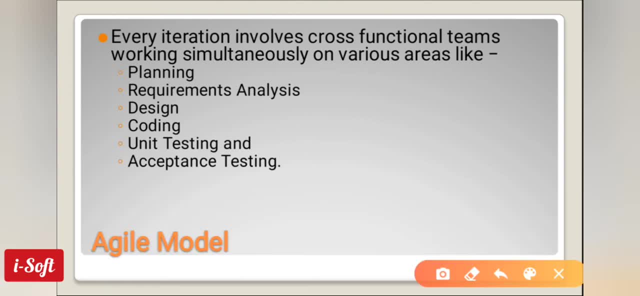 teams working simultaneously on various, various steps. so these are the steps that we have discussed in HDLC also: planning the requirement, analysis, design, coding, unit testing and acceptance testing means these steps are followed for development, and this each team will, or a many teams will, be included, or 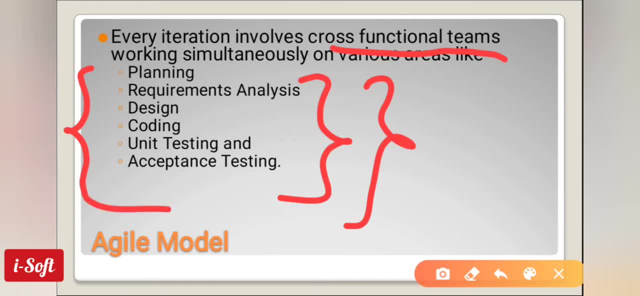 these are. they are included in various steps of the product development. so every iteration involves all these steps, starting from planning, requirement analysis, design, coding, unit testing and acceptance testing. so each iteration involves these all steps and working simultaneously, all teams are working simultaneously on these, each of the step. so this is the 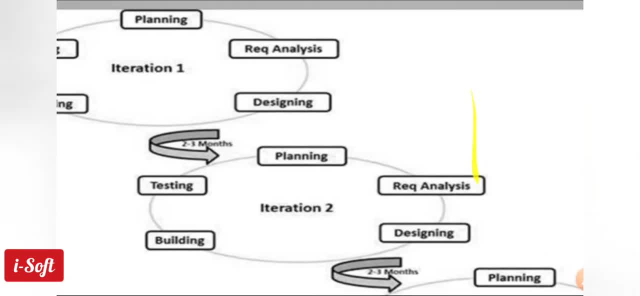 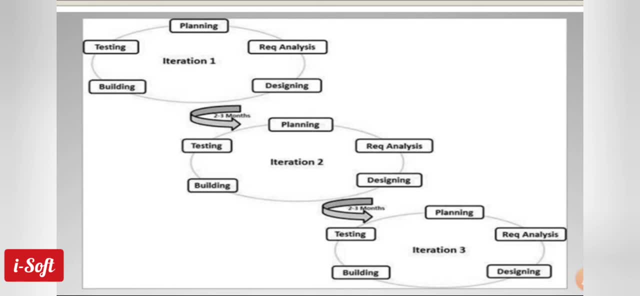 diagram that we can consider for agile development. so here diagram is very simple. you can see that the all steps are arranged sequentially and they are completed. and this is first iteration. then again all steps are arranged sequentially, they are completed. this is second iteration, then third iteration, and so on up till until we will get the complete product. so these are. 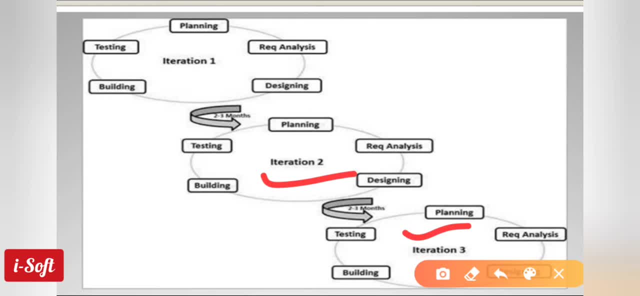 iterations. that are what we have discussed previously. so in each iteration all steps are included. you can see these steps are HDLC steps, that is, software development phase step and each iteration is having all these steps and each iteration will take two to three months or some weeks to complete the 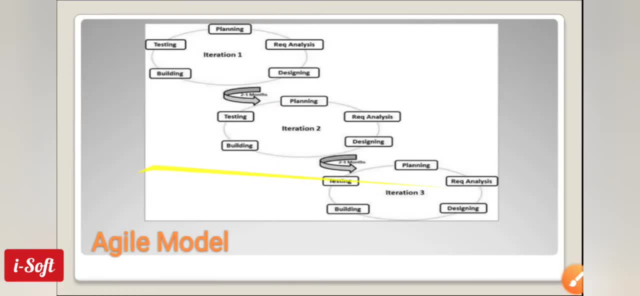 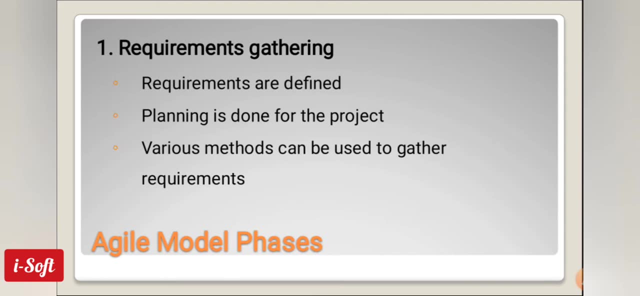 development of products. so diagram is very simple. you can understand just by looking at the diagram what it means. these steps are HDLC steps. then we will go one by one in each iteration. these steps are similar. so what are these steps? first step is requirement gathering. all these 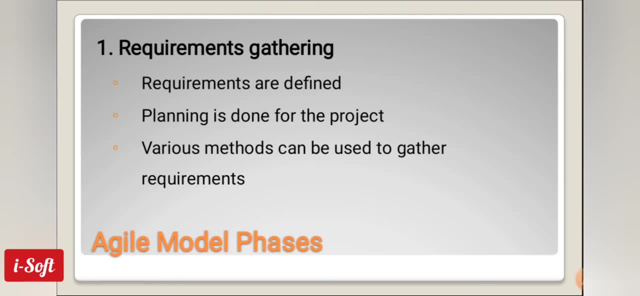 states we are discussing as DLC also. I am just explaining it in short: requirement gathering. in requirement gathering, requirements are defined. so these requirements are defined, then planning is done for the project. then planning is done for the project means these requirements are gathered from the customer. then according to that, requirements or overall planning is considered and all overall planning. 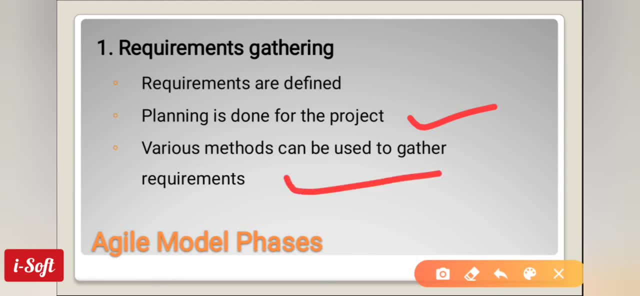 is developed, then various methods can be used to gather requirements, as we have discussed in waterfall model also, various methods can be used to gather the requirements means we can visit the. we can visit the business area for development or for gathering the requirements, or we can have question answer format, or we can provide different forms to the customer and we can gather the. 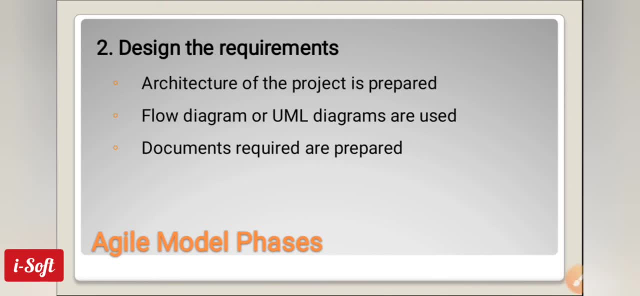 requirements for our project or software. then after gathering the requirements, then we will perform design part. so architecture of the project is prepared. in this step, by using flow diagrams or uml diagrams, we can perform design part and we can decide how the software will look and what is the architecture. 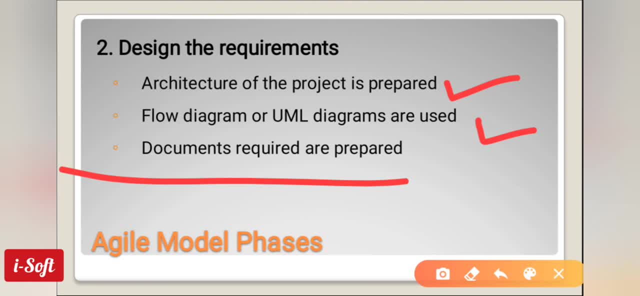 of software and various documents are prepared, for example, dds document, that is, design document specification, design specification document will be prepared, or different documents are there that are prepared for in this design and requirement step. then third step is: these steps are similar to sdlc, hence i am. 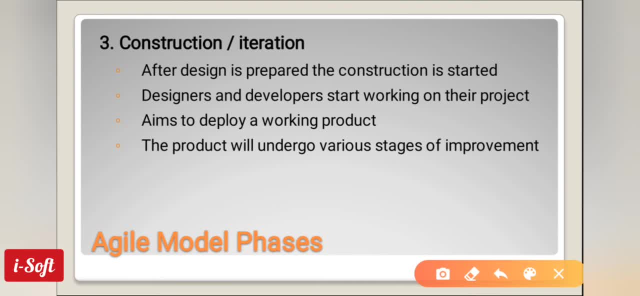 you explaining it in in fast. so, uh, construction and iteration is the next step. so after design is prepared, the construction is started. construction means construction and iteration means the implementation part. so implementation is started as soon as the design is ready. so after design design is prepared, the construction is started, designers and developers start working on their 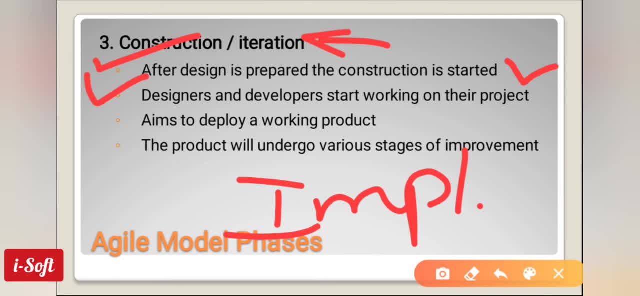 project and they will start developing the codes for the project. so it aims to deploy the working product means it aims to deploy the working product which is tested already to the customer. then product will undergo various stages of improvement. so in each iteration the coding is continuous process until and unless all the 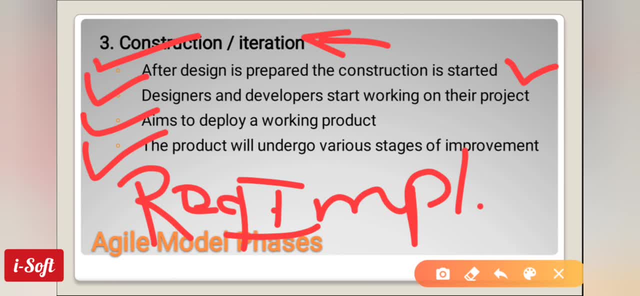 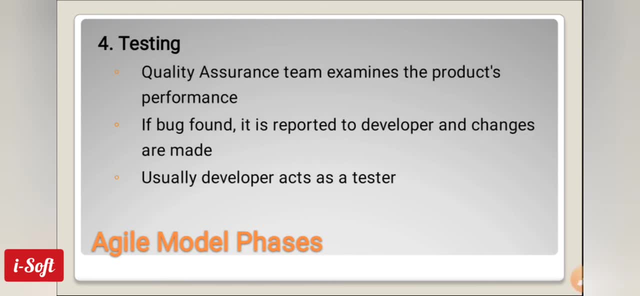 requirements are satisfied, so it focus on the requirements, so all the requirements. if are not satisfied, then this is the continuous process until and unless the requirements are satisfied, then after coding, the next step is testing. so in testing, quality assurance team will examines the product performance and if bug is found, it is reported to the developer and 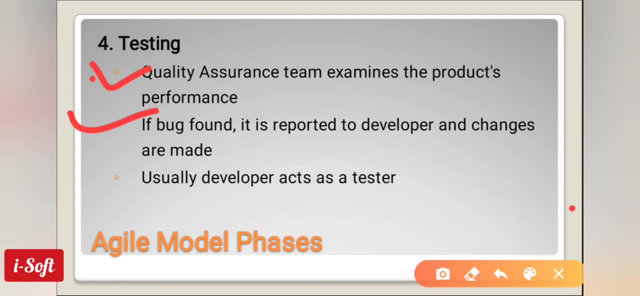 changes are made according to the report and usually developer acts as a tester. so in many software development project usually if developer is itself a tester, then many project usually developer is itself a developer wardrobe owner test thing. So in many software development project usually developer is itself a. 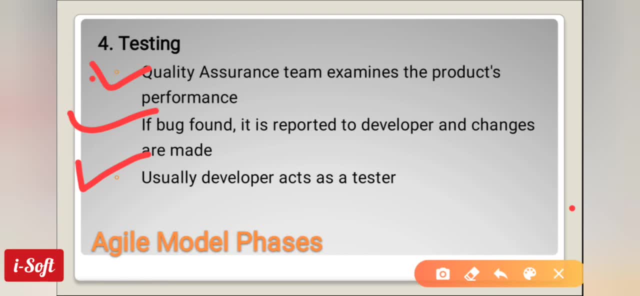 tester, So developer will test the module or the software part which is developer in a single iteration and the testing is performed by the developer itself. So what type of testing we will perform? We will perform the unit testing or we will test the module or build which is. 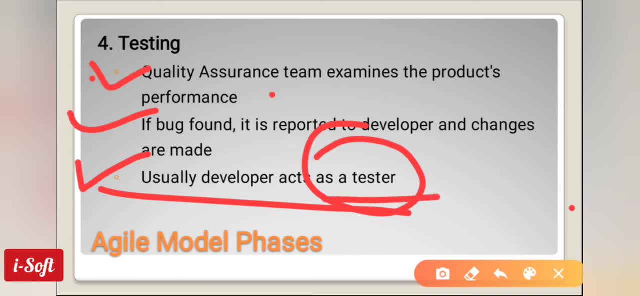 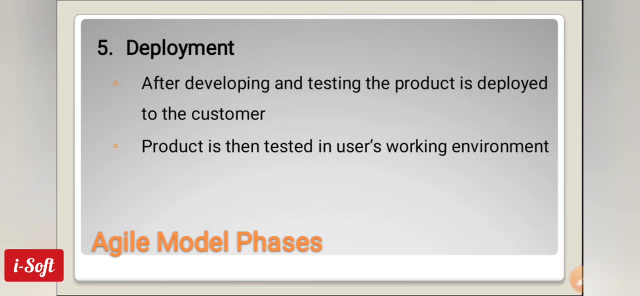 developed. So this testing team will be there sometimes, or sometimes. usually, developer acts as a tester. The next, after testing, deployment of the software: software: developing the software. the software is deployed to the customer. Which software? The tested software. After developing. 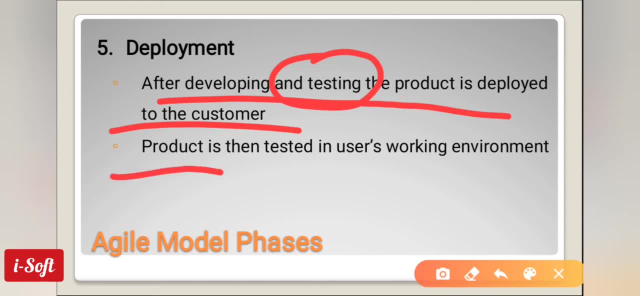 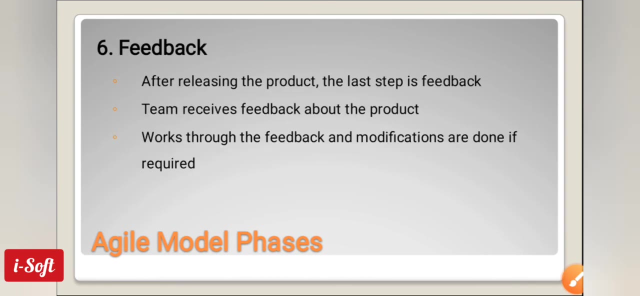 and testing. the software is deployed to the customer and product is then tested in user environment. So deployment means delivering the software to the customer which is already tested, and it will be also tested by the customer in their working environment. So, users, working environment, Then after testing, after delivering that software, 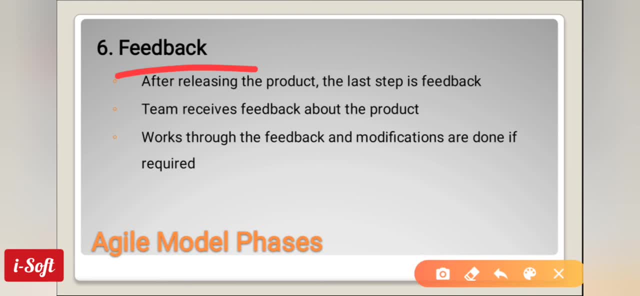 then feedback is taken from the customer After releasing the product. the last step is feedback. team receives feedback about the product and the team will work on this feedback And if modification are required then that modification allows the development. Then that modification is done by the team or by the developer. So, feedback afterもつ们, feedback after getting 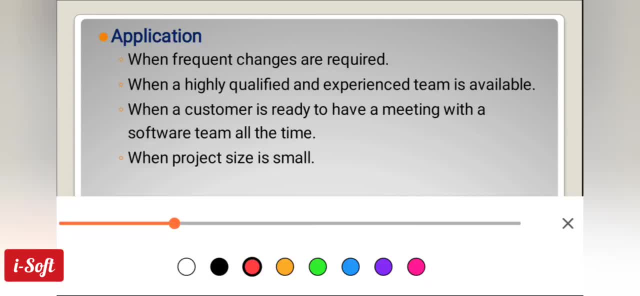 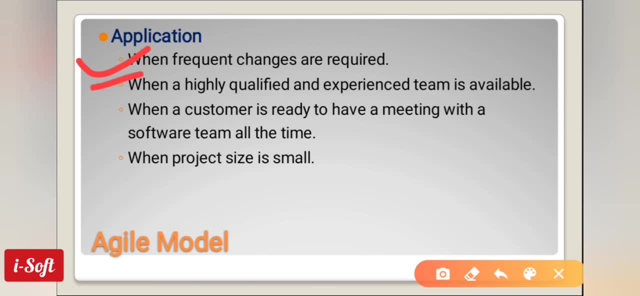 continue the software development if changes are required. So, as we have discussed in waterfall model also, applications: what are application? when frequent changes are required, when a highly qualified, experienced team is available, when customer is ready to have meeting with a software team all the time- means customer is available all the time- and when project size is small and 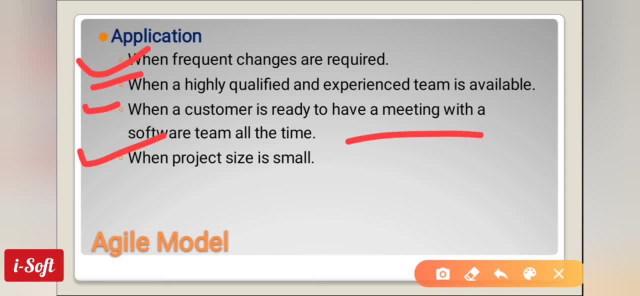 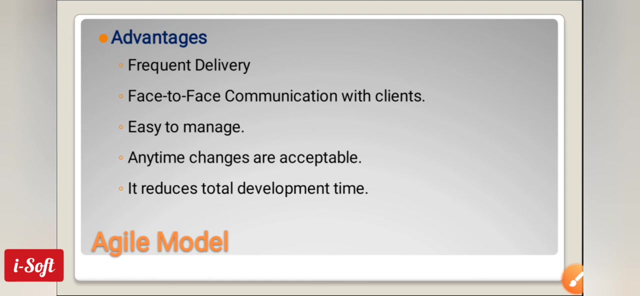 within short duration. we require the complete product. then we will use the agile model. So what are applications of agile model? simple, frequent changes are required, highly qualified team is available, customer is ready for meeting every time and product size is small or rapid development is required within short duration of time. So next advantages: advantages, what are? 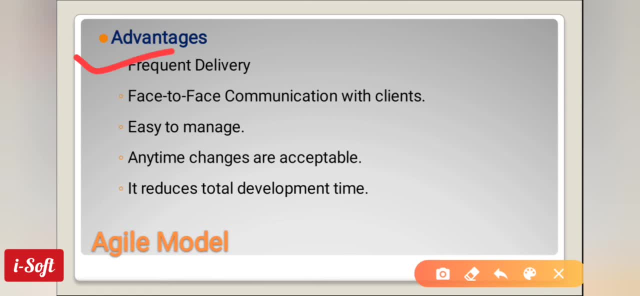 advantages of this agile model. frequent delivery means within short duration we will deliver to the software to the customer. Then frequent delivery means within short duration we will deliver to the software to the customer. Then we will have a face to face communication with clients or customer easy to manage. we will.